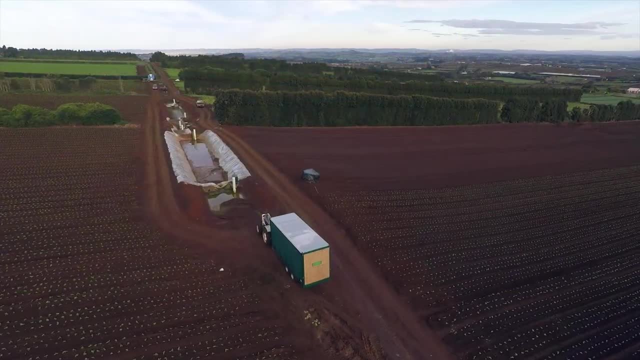 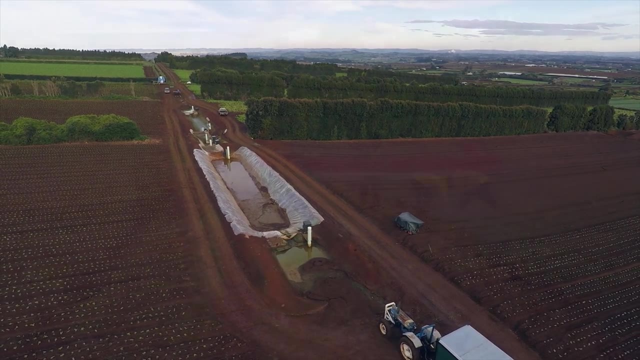 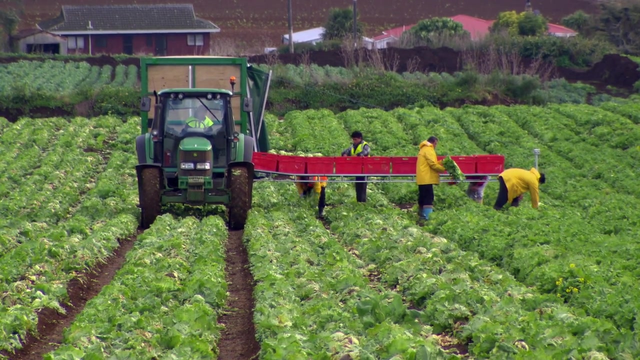 how much erosion is happening on properties, and then how much can you capture in sediment control devices? Our focus in this project is looking at the vegetable industry. Cultivated land obviously has erosion issues, and so then, how do you minimise erosion on a cultivated? 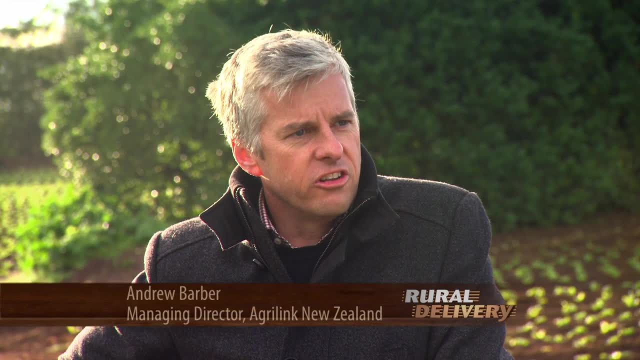 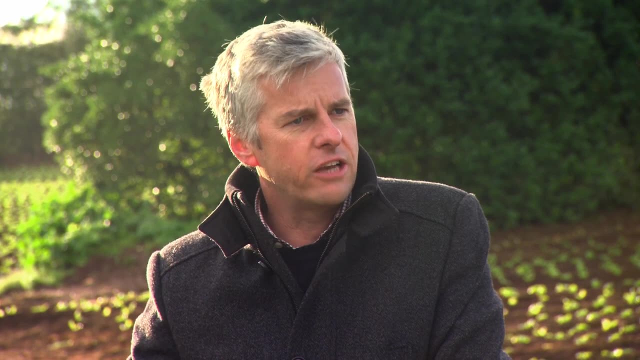 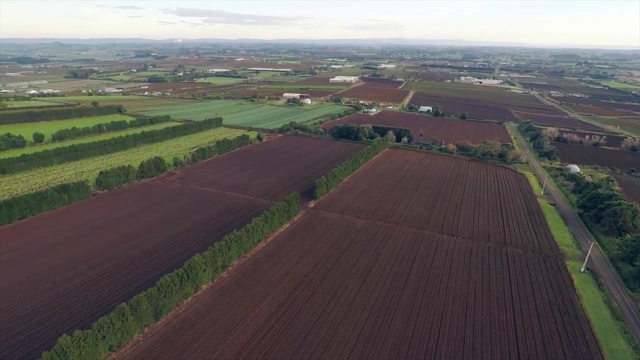 vegetable property. What's nice about this project is it builds on a massive amount of work that's been done previously. So back in the early 90s there was a really large storm event that occurred in Pukekohe and that really galvanised everybody to get involved in a project that looked at a whole 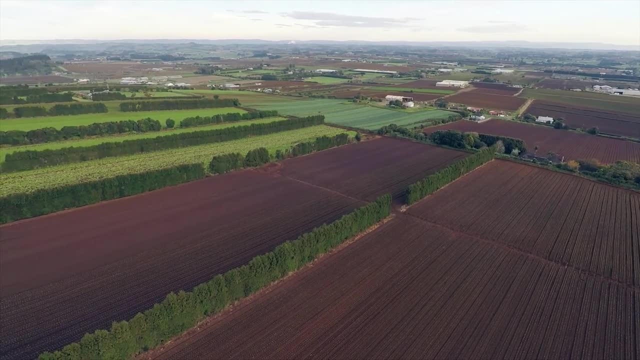 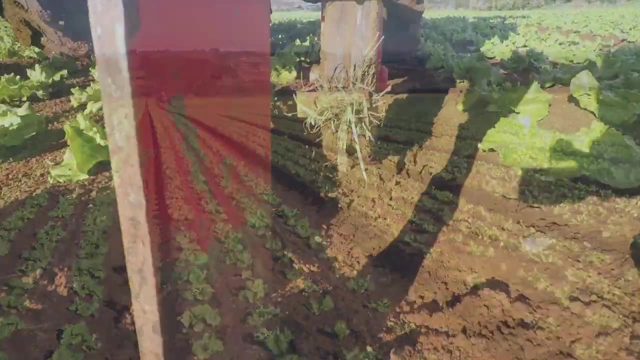 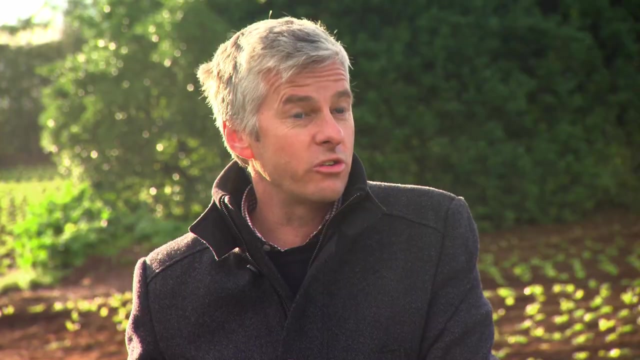 range of sustainability issues. One of those key issues was erosion and sediment control Amongst irrigation management, plant health, but erosion was what that project lived and died on. That project was the Franklin Sustainability Project, and it was a project that was really 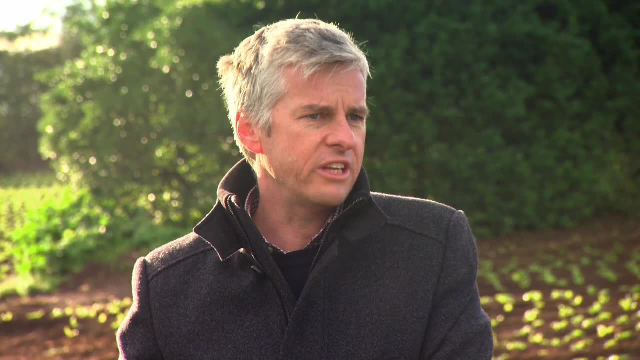 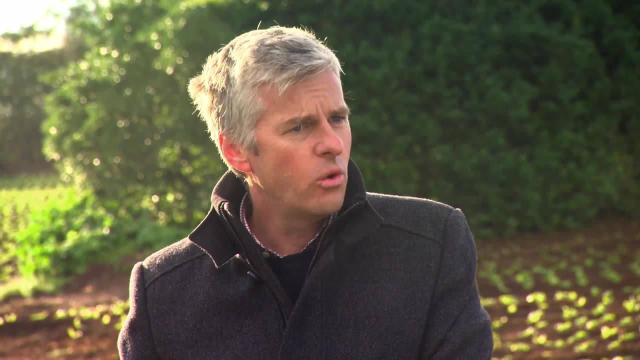 able to idealise Basil中, and so Far West also claimed that this was the right project. It's a fantastic example of getting a whole group of growers together, the council and coming up with a whole range of sustainability measures. The nice thing about that was you. 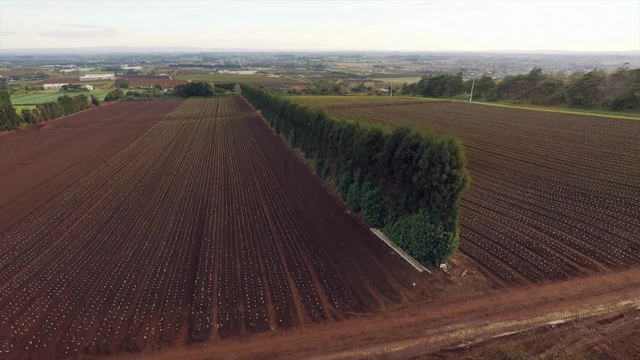 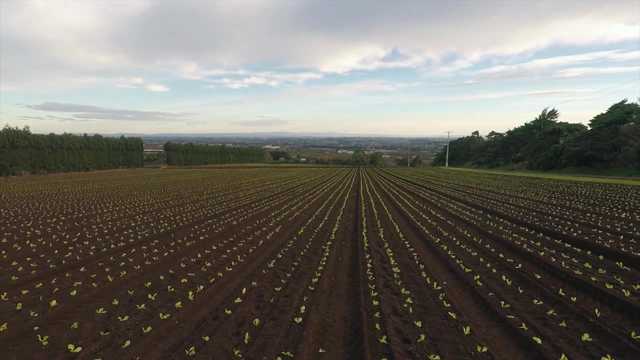 have everybody coming together rather than splitting off and doing whatever they thought was the best solution. People need to have the numbers and the details, and that's what this most recent project is all about. How do you quantify what's happening in the measures that the growers have put up 11 00 suits cost maógou: 1 00 suits. Environmental Change, supposed to casa 1 00 suits to solitude in over 1 000 sa��. 11 00 suits, equal needs andregistrable needs, which is what the project did: 11 00 suits situations. 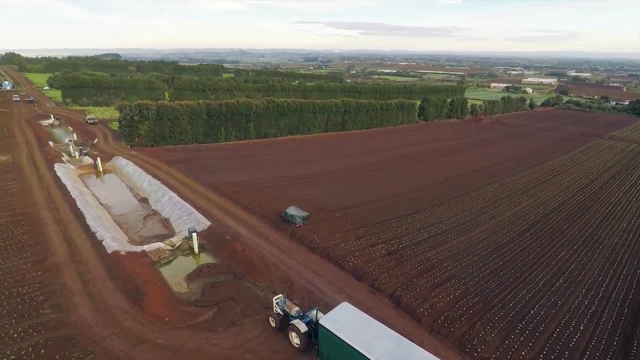 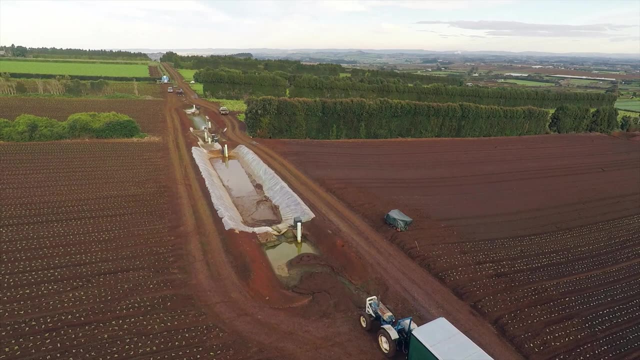 and urban areas that went to the different local eras- 12: 00, which was around Mic, erlebes and elixir values- need to have sediment control. Our issue with sediment control is there's two key elements. First of all, there's bed load, which is the really heavy stuff that drops out quite quickly. 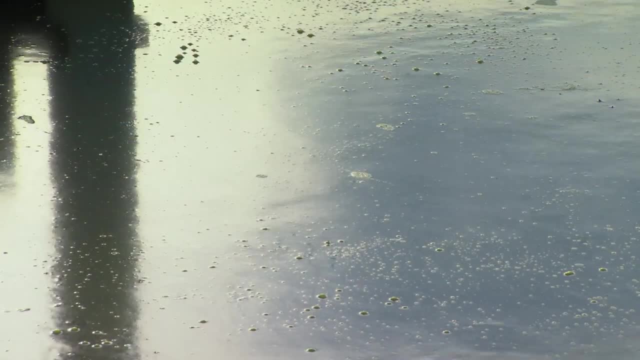 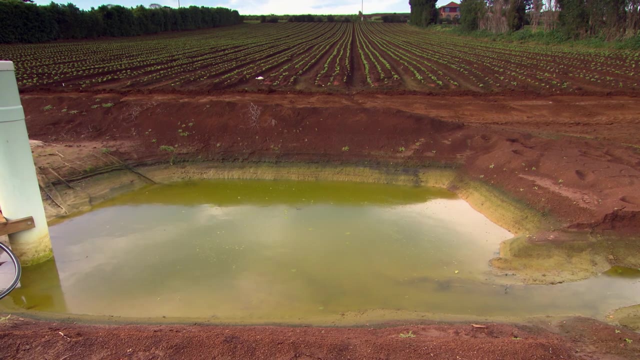 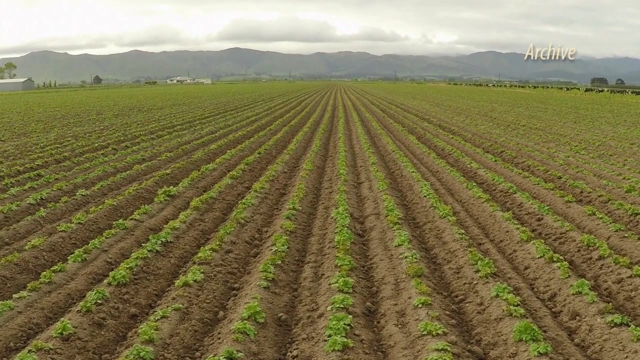 The second element is suspended sediment, and it's the suspended sediment that gets into the waterways that causes a whole lot of issues downstream. This project has had a number of trials that have run. One of them was in Levin, where we looked at the size of the riparian strip. 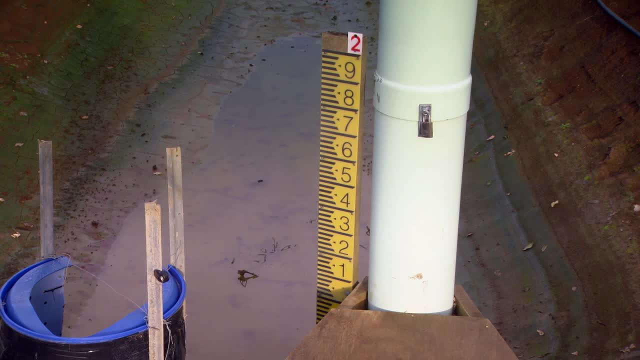 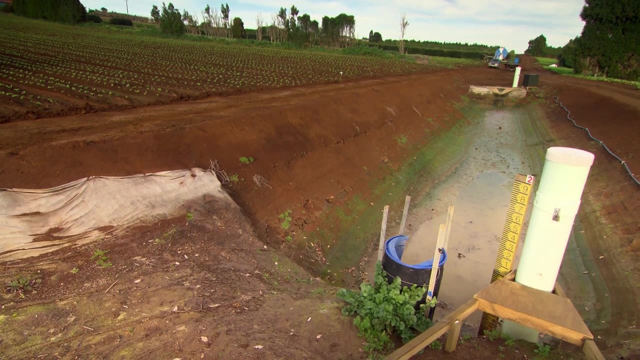 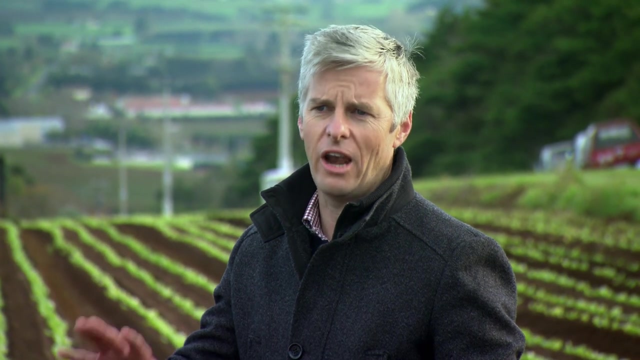 and in Pukekohe, our focus has been on sediment control. So what is the effectiveness of a silt trap and how big a silt trap do you need to be effective? We have a four-step process when you look at a paddock. So the first step is: what is my paddock? how large is the paddock? what's the slope? 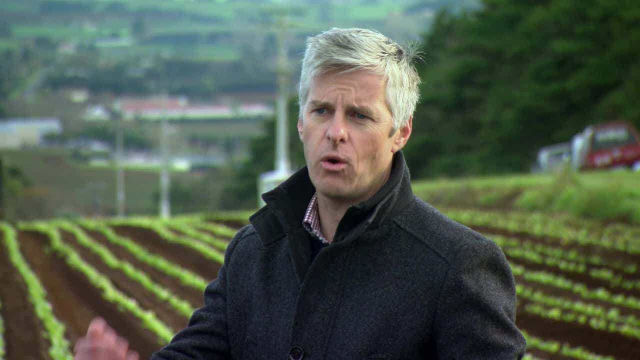 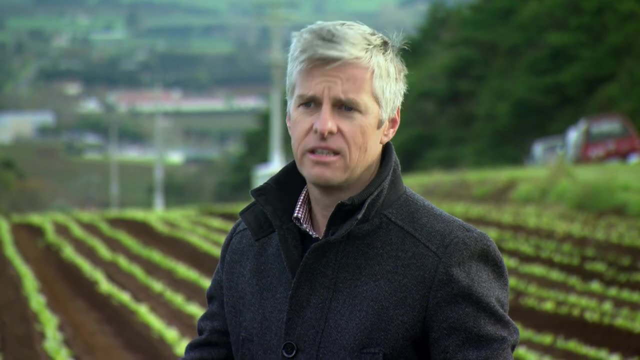 That's my paddock assessment. Step two is: how do I minimise the water that enters that paddock, so that way you only deal with the water that directly falls on the paddock. Step three: how do I deal with the water that does fall on the paddock? So that's erosion control. 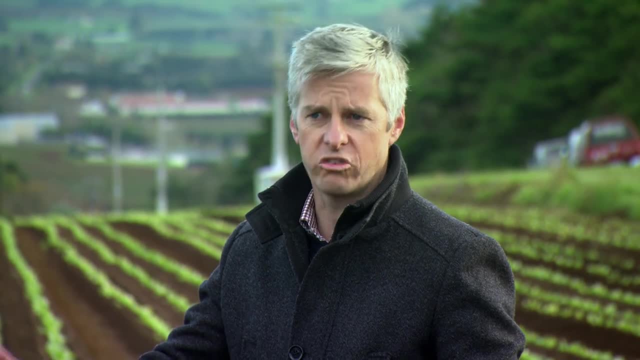 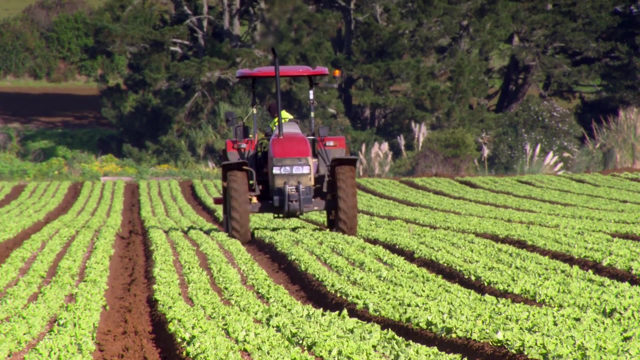 What do I do in the paddock? Do I have cover crops? Do I do wheel track ripping? What am I doing in the paddock to stop that saw from moving? The fourth step is sediment control. So what do I need to do to stop the water that leaves the paddock having lots of sediment? 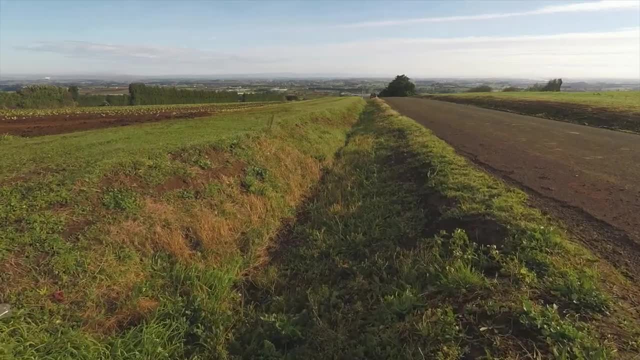 in it. Ie: do I need a silt trap? Do I need an earth-bound? That's my final step. This is the stuff that's going to be the main section of the paddock. This is the part where the sediment is going to be the main section. This is the stuff that our 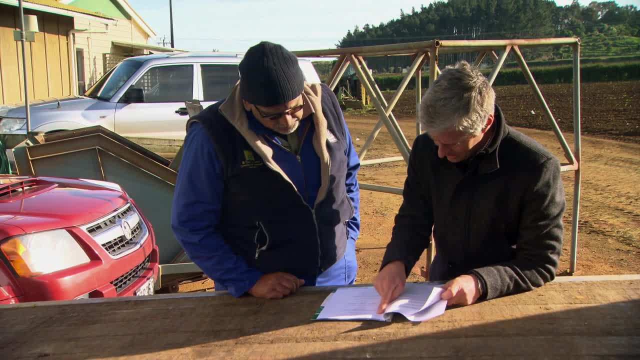 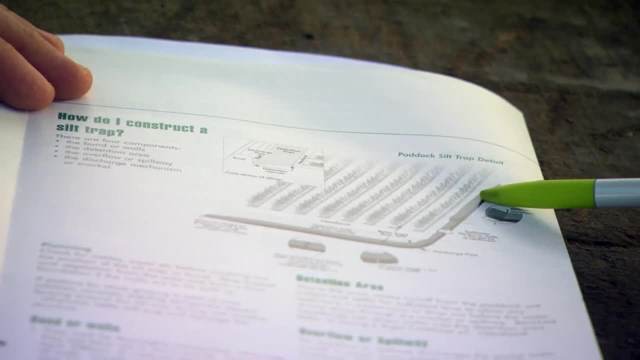 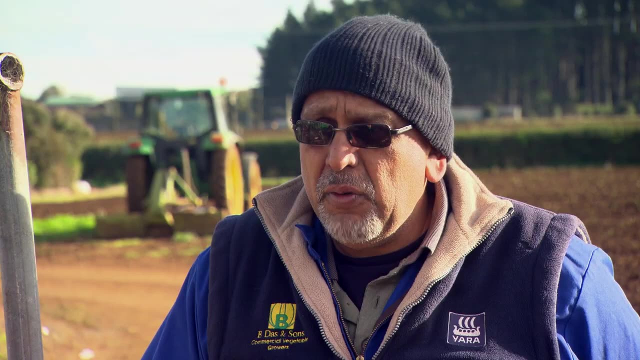 you want to look at, Eric, The whole paddock assessment. What we've done over the years now is bunding on the headlines silt traps and wheel track ripping and that minimises- not totally eliminates it but- soil erosion. In the winter time we put cover crops in. 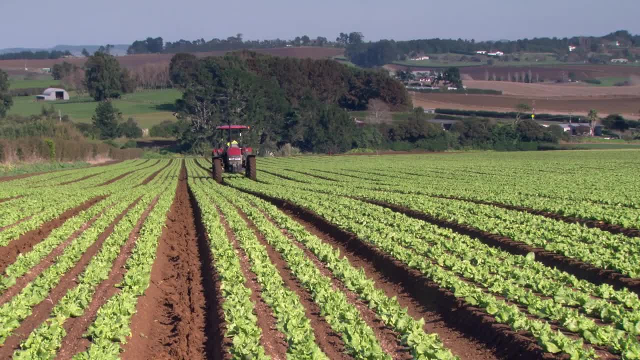 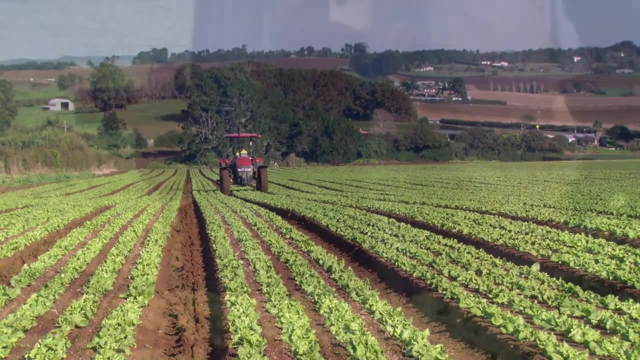 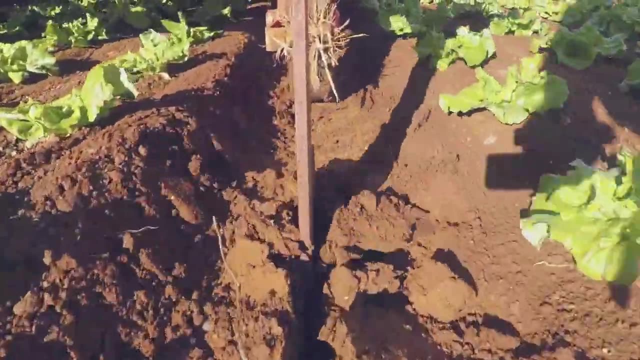 and that holds the soil in place. at times The tracks are panned over the summer time or when you work the ground and the water can't drain freely. so with the wheel track ripping it opens up a little v and lets the water drain in and soaks away. in theory It's working on slopes up to 15. 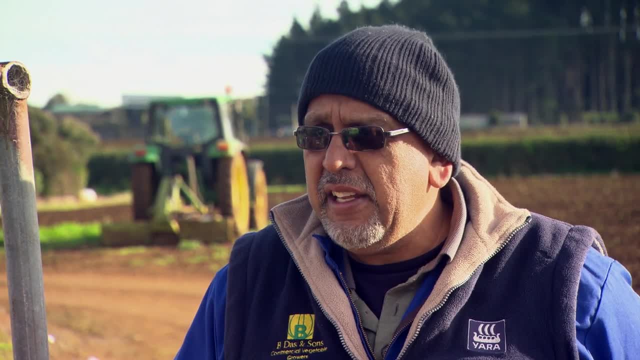 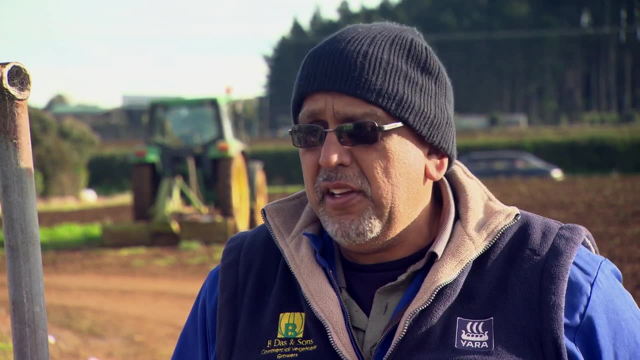 degrees On heavy downpour, you can actually encourage that soil movement. so you've got to pick and choose which paddocks. you do it By loosening up the soil on a two to three inch rain downpours. it will move. It has its advantages and has its disadvantages also. 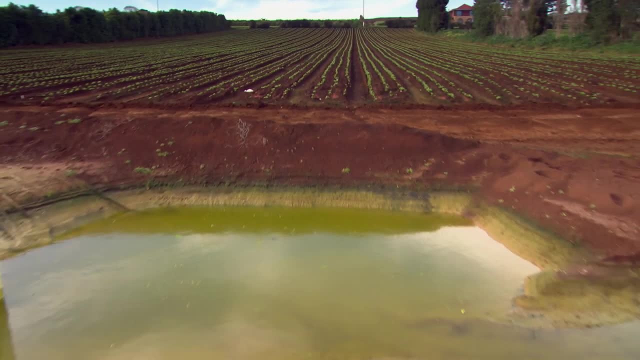 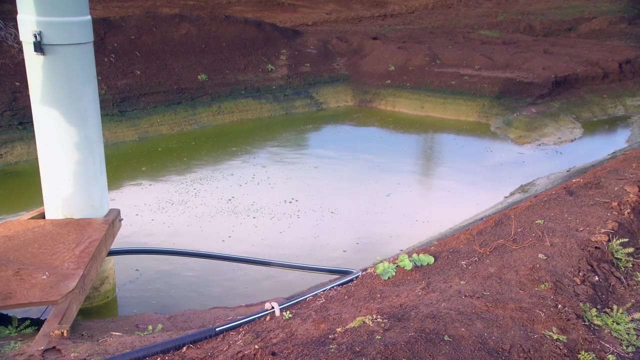 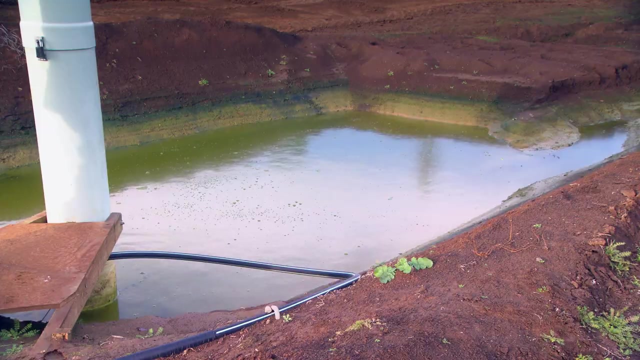 What we have here is a forebay, and the forebay is before it goes into the main silt trap. The idea of a forebay is it's much, much easier to clean out. You can get into a forebay much easier than you can get into a silt trap. What happens in the forebay is the bed load drops out super fast. So